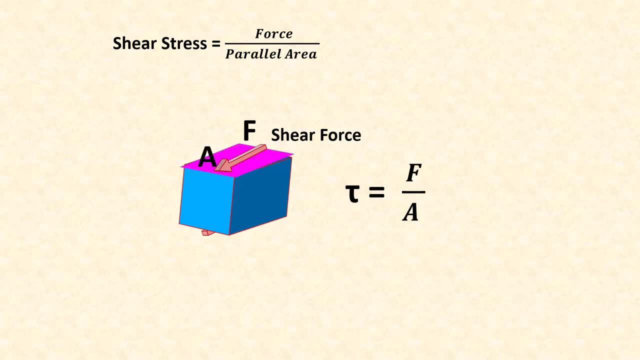 Compressive stress notation is generally σc. Shear stress notation is generally σt. Shear stress notation is generally σc. See this example: Tensile force is 10 Kilo Newton. Tensile force is 10 Kilo Newton. 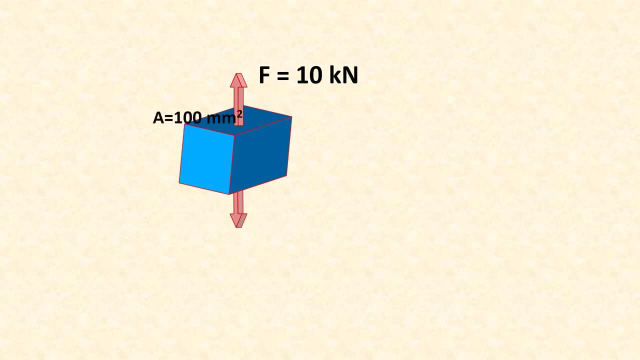 Area is 100 mm. Area is 100 mm, then tensile stress Sigma T is equal to 100 Newton per millimeter square or 100 mega Pascal. strength: ability of the material to withstand and apply stress. generally maximum stress withstand without failure: see this example. 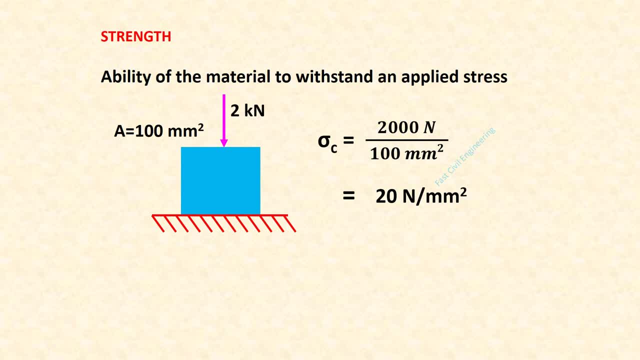 compressive force: 2 kilo Newton area: 100 millimeter square. therefore compressive stress: Sigma C is equal to 20 Newton per millimeter. now change the force as 5 kilo Newton. then Sigma C is equal to 50 Newton per millimeter scale: now force is 10 kilo Newton. Sigma C: 100 mega Pascal: now force. 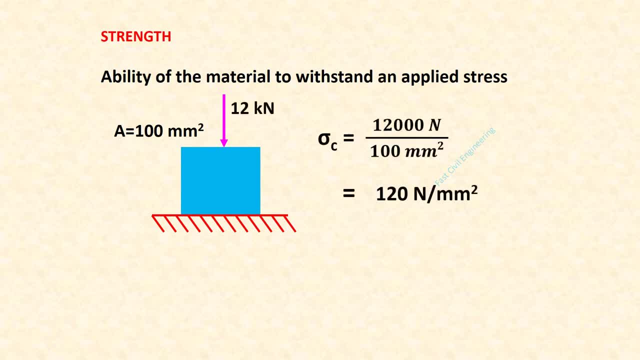 change as 12 kilo Newton. Sigma C is equal to 120 mega Pascal, Civic Mega Pascal. now force applies just greater than 12 minonito failure occur. that is a Sigma setting off password. sigma max, 120 mega Pascal. we can see sleep of this. meant to be at least 100. 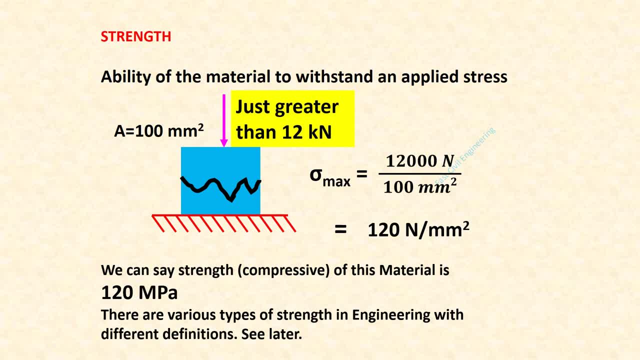 120 mega Pascal. there is actually compressive ten. we can say here 10- 20 mega Pascal. actually compressive strength 600 was 살�re four and 10- 120 MPa. There are various types of strength in engineering with different definitions. 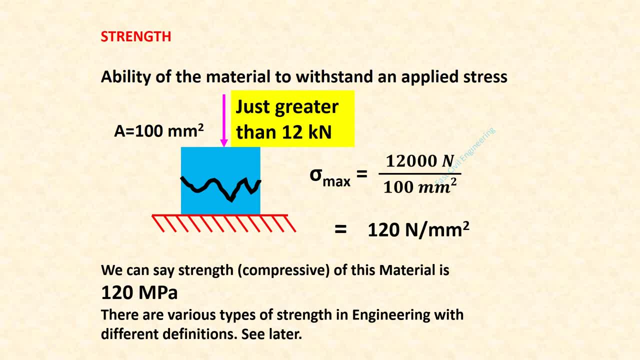 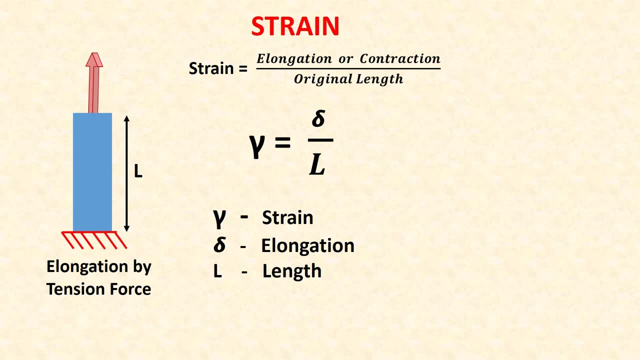 See later. Strain Strain is equal to elongation or contraction over original length. Gamma is common notation for strain. Gamma is equal to delta over L. Delta is elongation L original length. Strain by compression force. Gamma is equal to delta over L. But delta is equal to contraction, not elongation here. 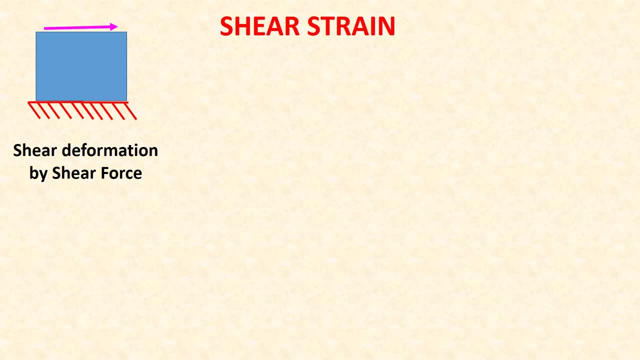 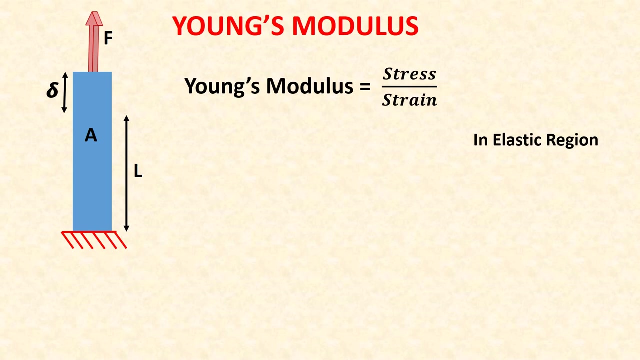 Shear strain. Young's modulus or modulus of elasticity. Young's modulus is equal to stress over strain in elastic region. Young's modulus notation E is equal to sigma over gamma. Young's modulus notation E is equal to sigma over gamma. Elasticity. 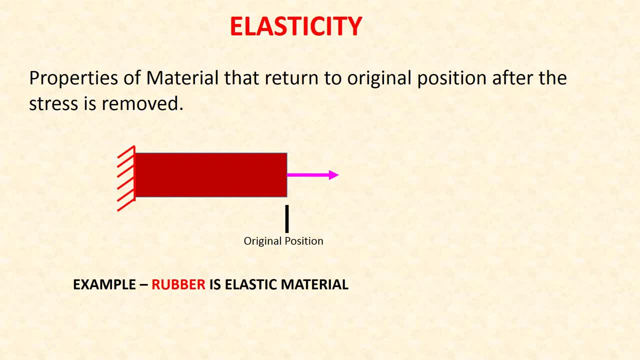 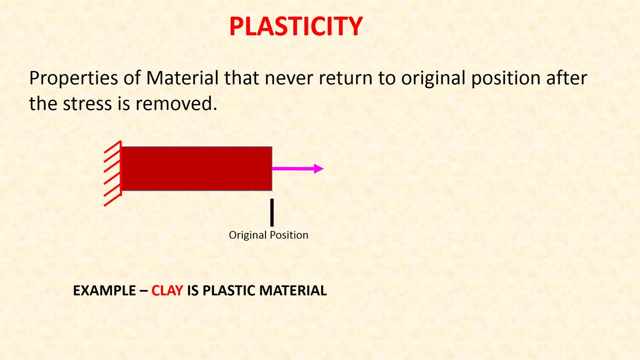 Properties of material that return to oil after stress is removed. Plasticity. Properties of material that never return to original position after the stress is removed. stress is applied, elongated. after that stress is removed, never return back to original position or partially recover. Clay is plastic material. 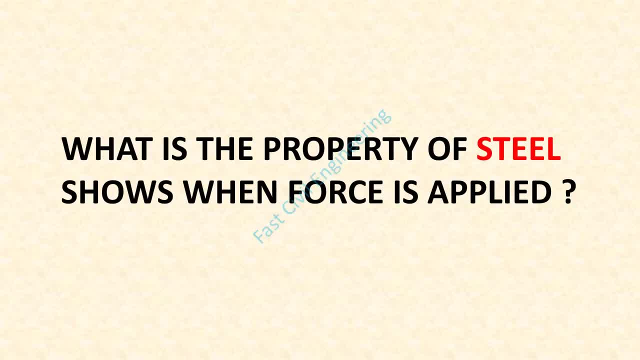 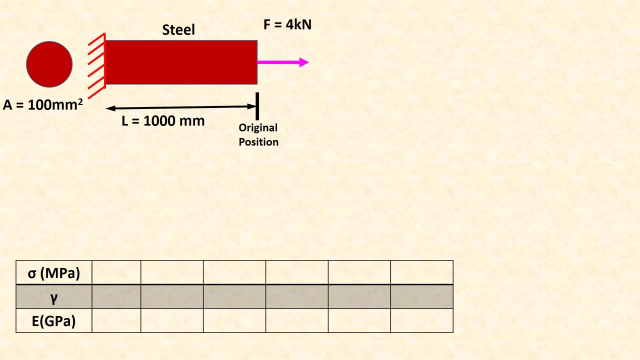 What is the property of steel shows when force is applied. Let us understand by good example. force applied: 4 kilo Newton steel is elongated by Delta E equal to 0.2 millimeter. elongation is 0.2 millimeter cross-sectional area. 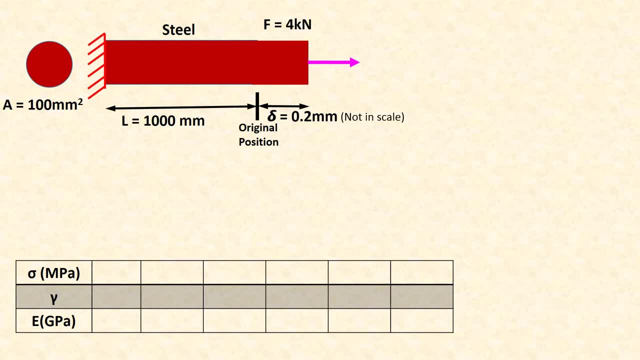 100 millimeters square. therefore, stress is equal to 40 Newton per millimeter square. strain gamma is equal to elongation over original length, that is 0.0002.. Therefore, Young's modulus stress over strain: 200 Giga Pascal. Now, when remove the force, steel is returned back to original position. 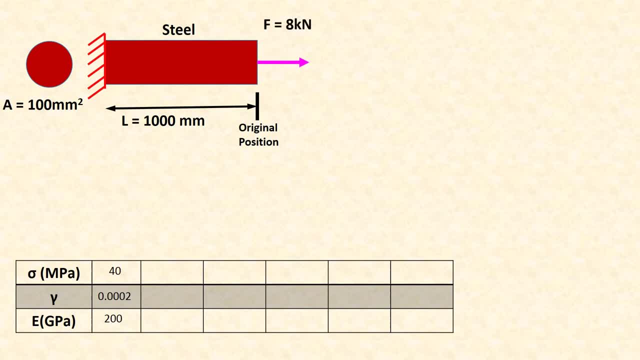 Now double the force. Force has 8 kilo Newton Elongation. also double Delta is equal to 0.4 millimeter. Again, Sigma: 80 mega Pascal. Gamma 0.0004.. Young's modulus: 200 Giga Pascal. 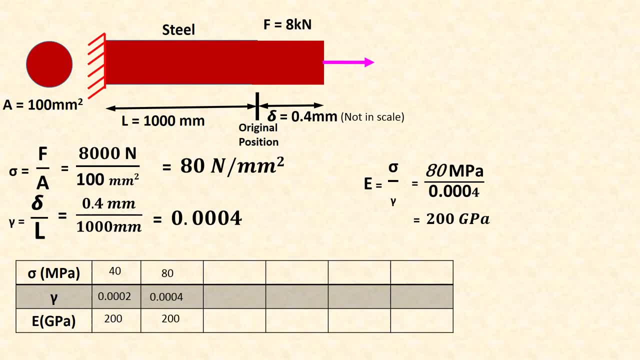 Same value. Remove the force: Return back to original position. Now, when remove the force, steel is returned back to original position Again. gamma: 80 mega Pascal Gamma: 0.4 millimeter. Again double the force. Force is equal to 16 kilo Newton. 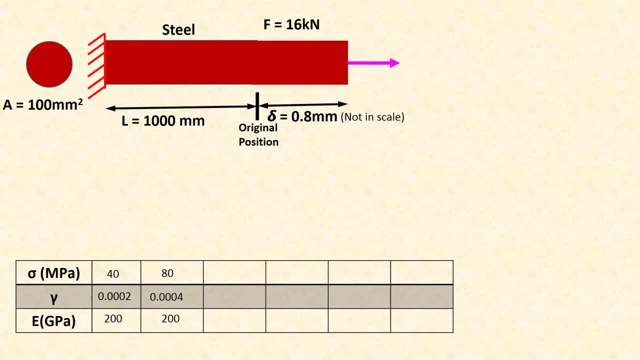 Elongation also proportionally increased. Delta is equal to 0.8 millimeter. Sigma is equal to. Gamma is equal to 0.0008. Young's modulus is equal to 200 Giga Pascal, same value When force is removed. return back to original position. 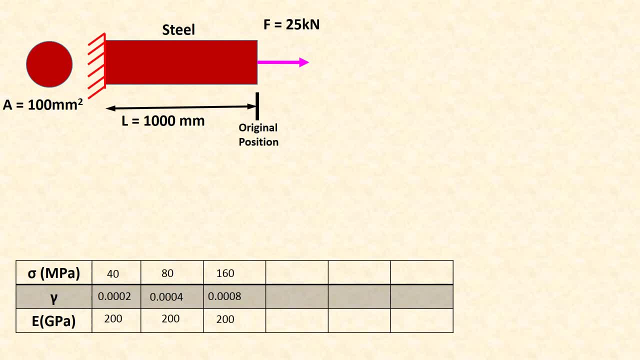 Force change as 25 kilonewton delta is equal to 1 millimeter proportional in interest. Sigma is equal to 250 Mega Pascal, Gamma is equal to 0.00125,. E is equal to 200 Giga Pascal. 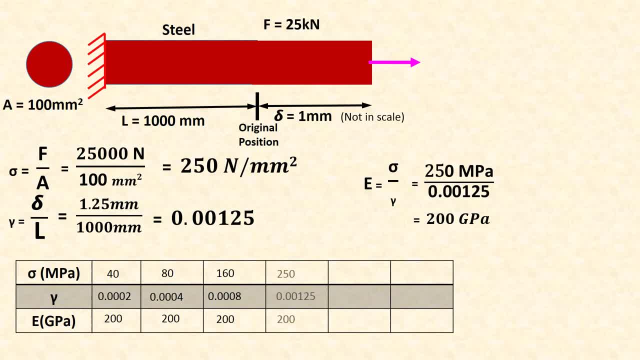 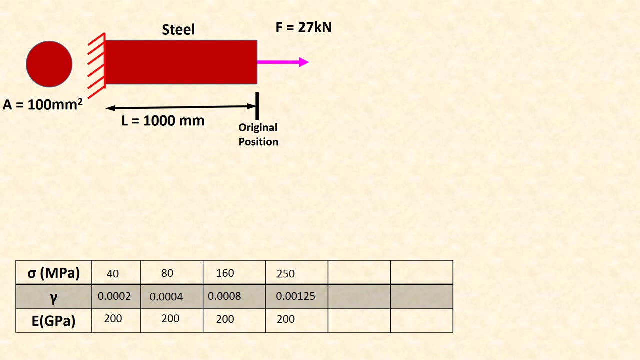 same value When force is removed. return back to original position. Now force increase as 27 kilonewton elongation, unexpected elongation. high elongation delta is equal to 5 millimeter. This is not proportionally increased, suddenly increased. Sigma is equal to 270 Mega Pascal, Gamma is equal to 0.005, Young's modulus is equal to 54 Giga Pascal. Actually, now steel is entering to plastic region. Young's modulus values only valid in elastic region. Now force is removed. never return back to original position. 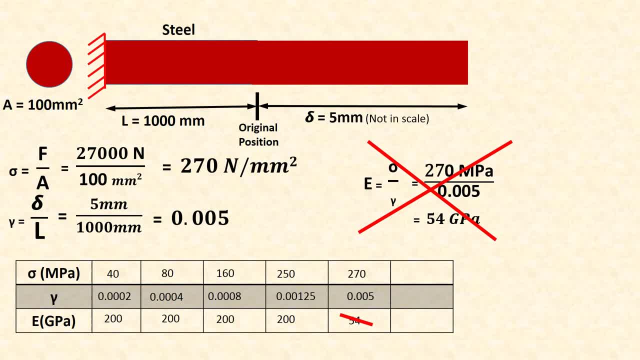 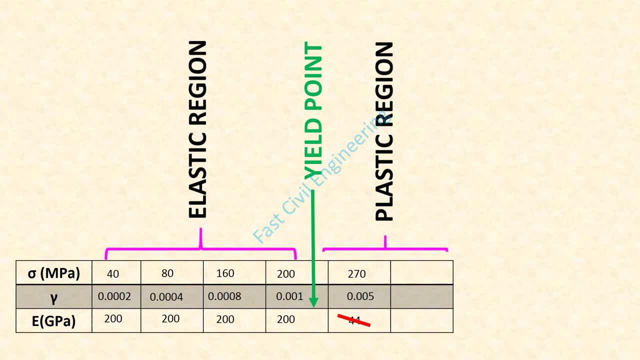 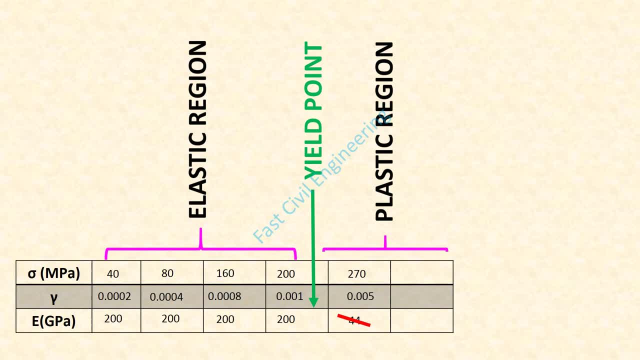 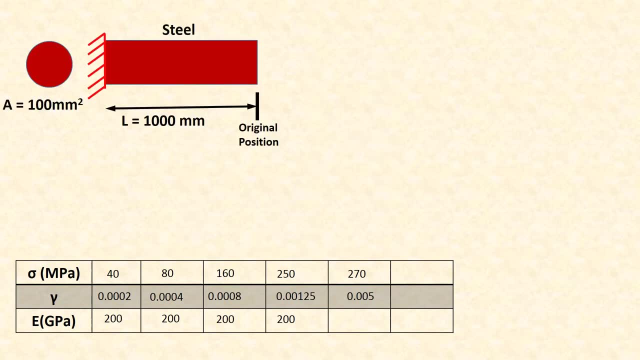 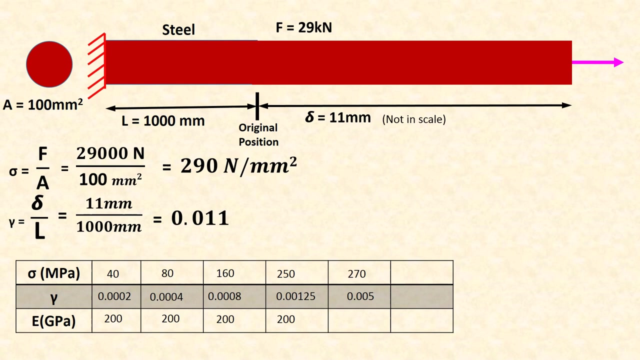 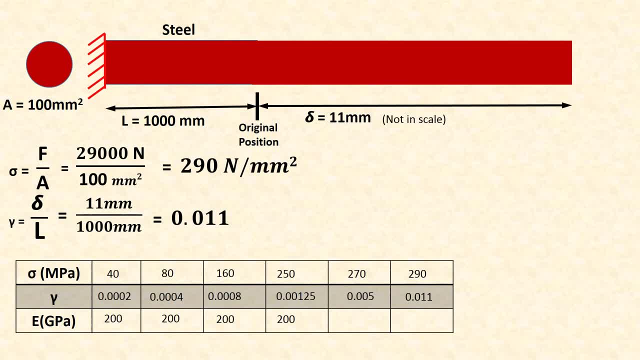 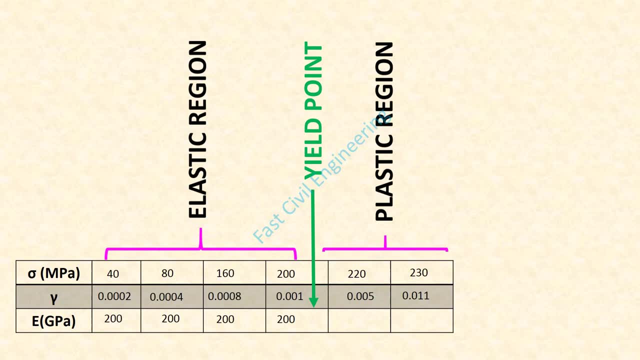 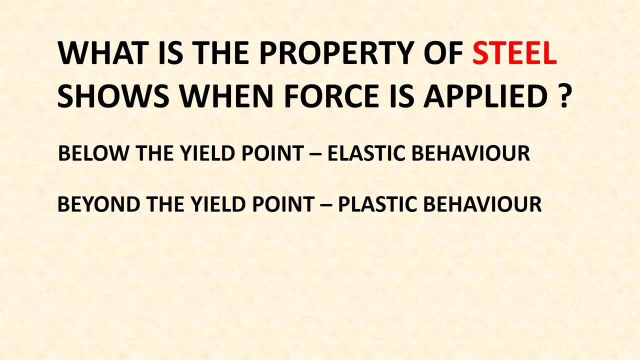 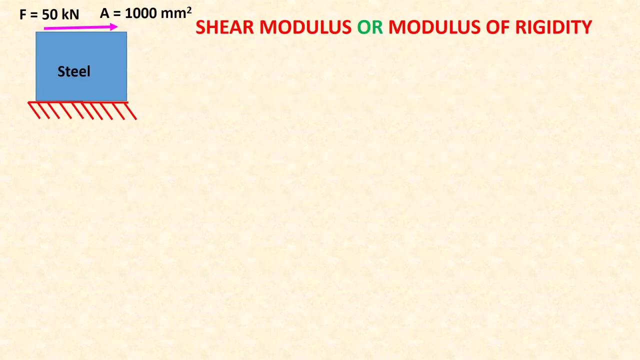 this state plastic region. what is the property of steel shows when force is applied. the answer is: below the yield point, elastic behavior. beyond the yield point, plastic behavior. the products are shear modulars. shear modulus modulus. new moisture g is equal to tau over gamma, example. shear stress. tau is equal to here 50,000 newton, because 50 kilonewton 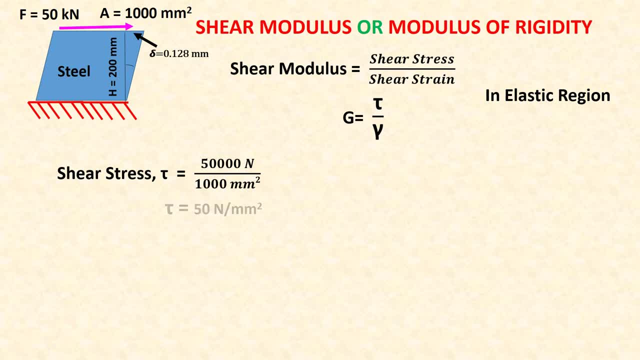 over 1000 millimeter square tau is equal to 50 newton per millimeter square omega. per square shear strain gamma is equal to 0.128. over 200 gamma is equal to 0.00064. therefore, shear modulus g is equal to 78 giga Pascal.